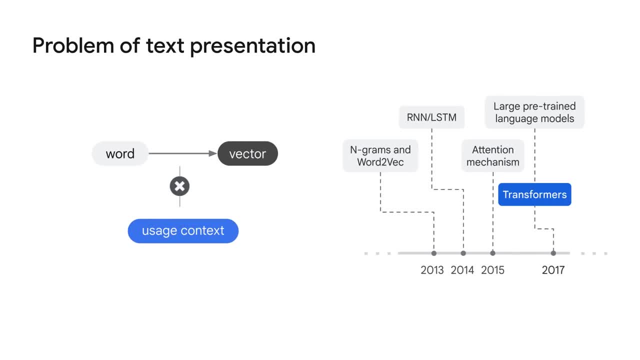 National Library of Congress in 2019.. The paper is titled Attention Mechanisms, and Attention Mechanisms is All You Need. Although all the models before transformers were able to represent words as vectors, these vectors did not contain the context and the usage of words. changes based on. 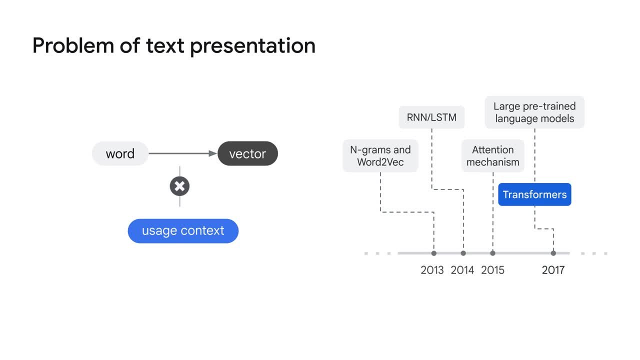 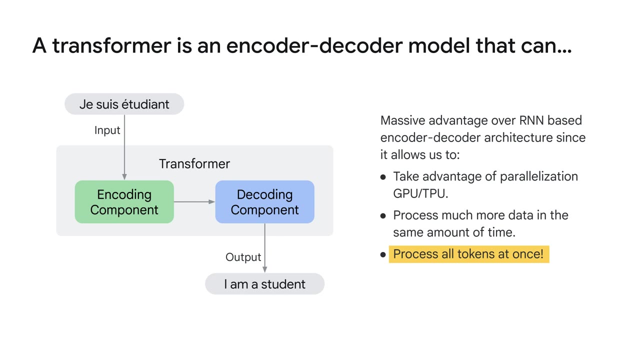 the context. For example, bank in riverbank versus bank in bank robber might have the same vector representation before attention mechanisms came about. A transformer, for example, might have. the Transformer is an encoder-decoder model that uses the attention mechanism. It can take advantage of parallelization and also process a large amount of data at the same time because of its model architecture. 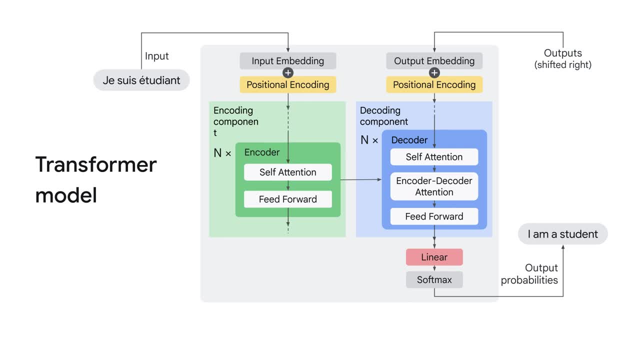 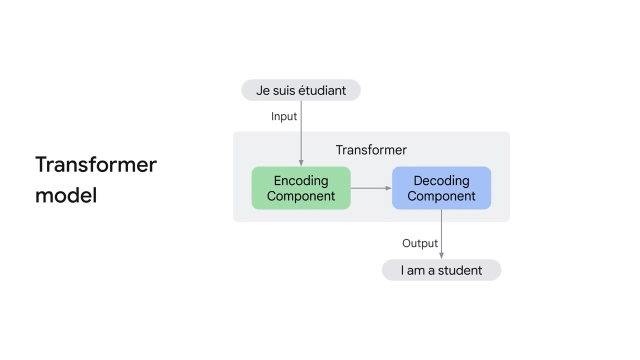 Attention mechanism helps improve the performance of machine translation applications. Transformer models were built using attention mechanisms at the core. A transformer model consists of encoder and decoder. The encoder encodes the input sequence and passes it to the decoder, and the decoder decodes the representation for a relevant task. 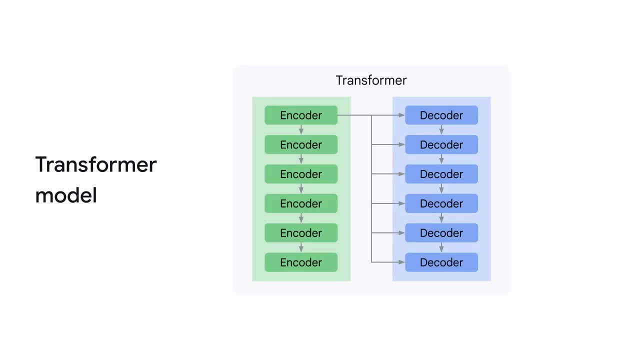 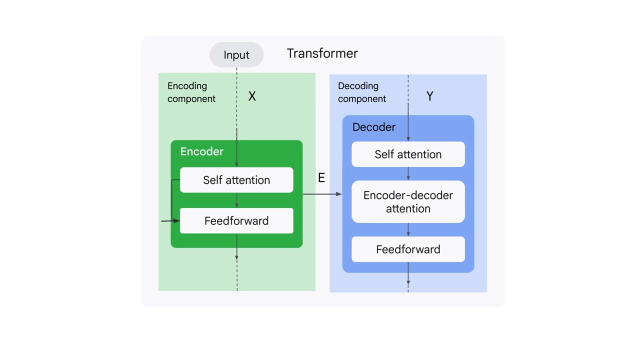 The encoding component is a stack of encoders of the same number. The research paper that introduced transformers stacks six encoders on top of each other. Six is not a number, It's just a hyperparameter. The encoders are all identical in structure, but with different weights. 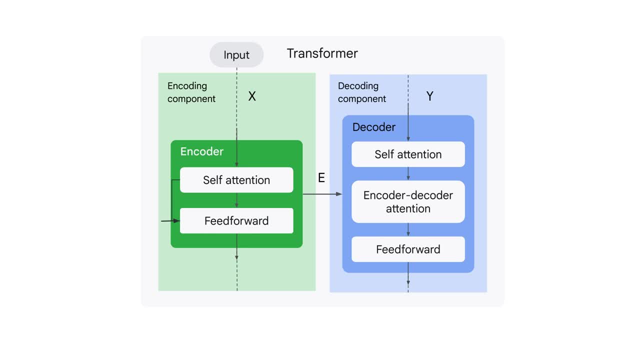 Each encoder can be broken down into two sublayers. The first layer is called the self-attention. The input of the encoder first flows through a self-attention layer which helps the encoder look at relevant parts of the words as it encodes a center word in the input sentence. 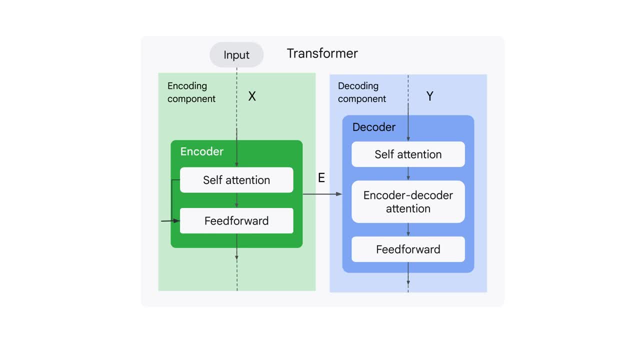 And the second layer is called a feedforward layer. The output of the self-attention layer is fed to the feedforward neural network. The exact same feedforward neural network is independently applied to each position. The decoder has both the self-attention and the feedforward layer, but between them is the encoder-decoder attention layer that helps the decoder focus on relevant parts of the input sentence. 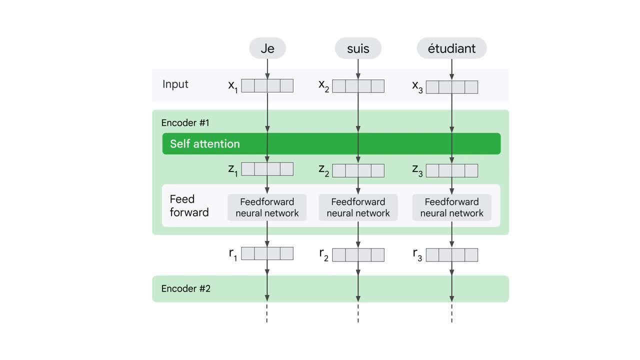 After embedding the words in the input sequence, each of the embedding vectors flows through the two layers of the encoder. The word at each position passes through a self-attention process, Then it passes through a feedforward neural network. The exact same network, with each vector flowing through it separately. 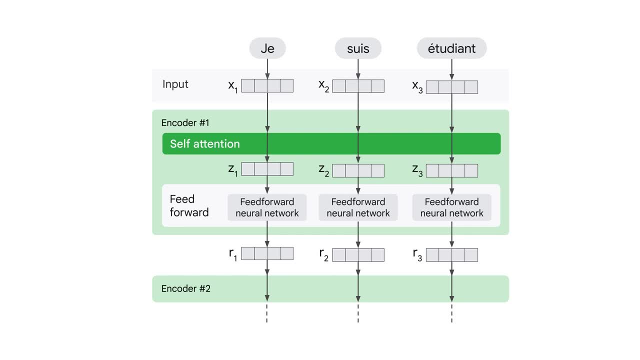 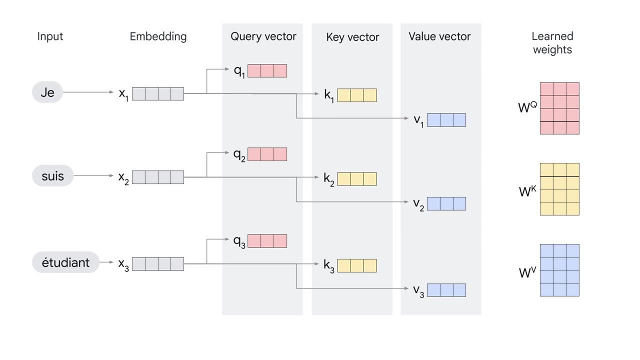 Dependencies exist between these paths in the self-attention layer. However, the feedforward layer does not have these dependencies and therefore various paths can be executed in parallel while they flow through the feedforward layer. In the self-attention layer, the input embedding is broken up into query key and value vectors. 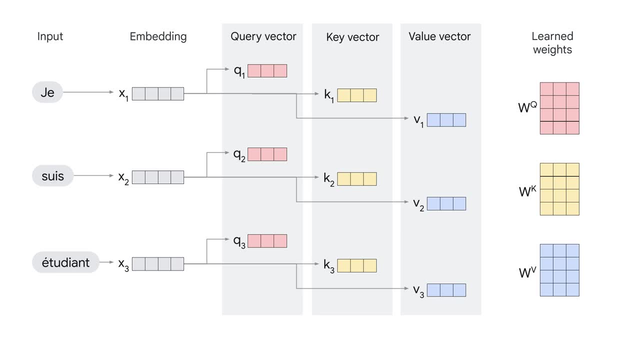 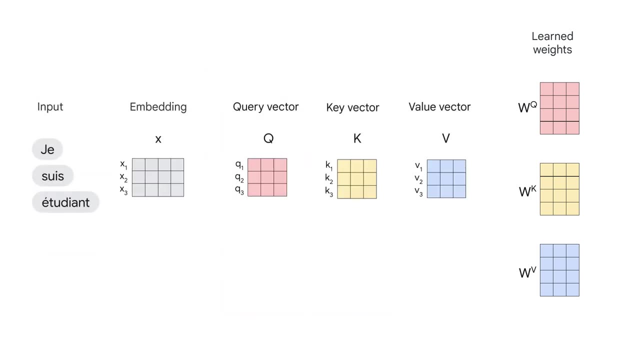 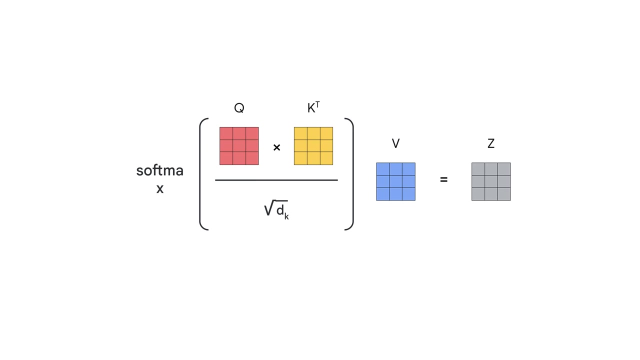 These vectors are computed using weights that the transformer learns during the training process. All of these computations happen in parallel in the model in the form of matrix computations. Once we have the query, key and value vectors, the next step is to multiply each value vector by the softmax score in preparation. to sum them up, 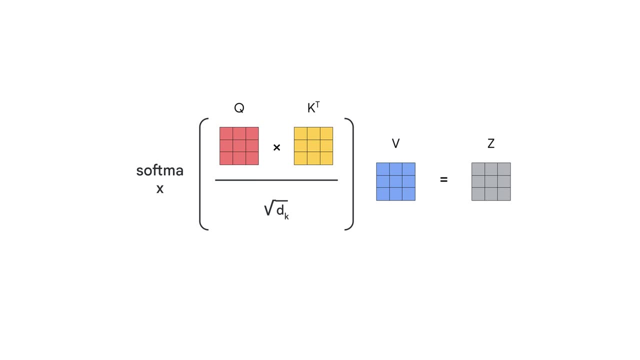 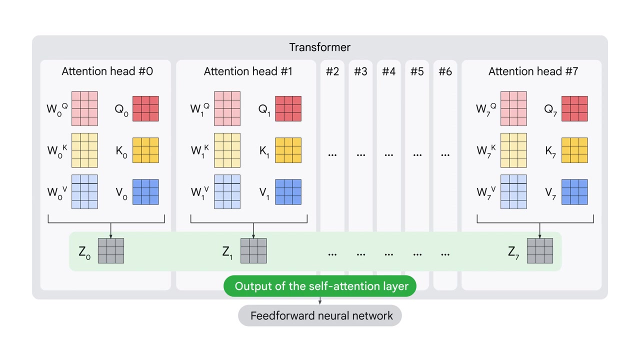 The intuition here is to keep intact the values of the words you want to focus on and leave out irrelevant words by multiplying them by tiny numbers like 0.001,, for example. Next, we have to sum up the weighted value vectors, which produces the output of the self-attention layer at this position for the first word. 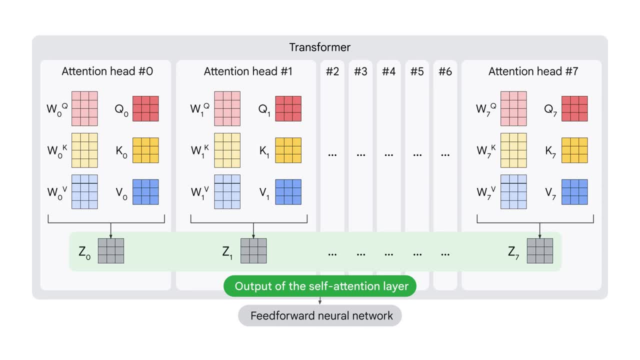 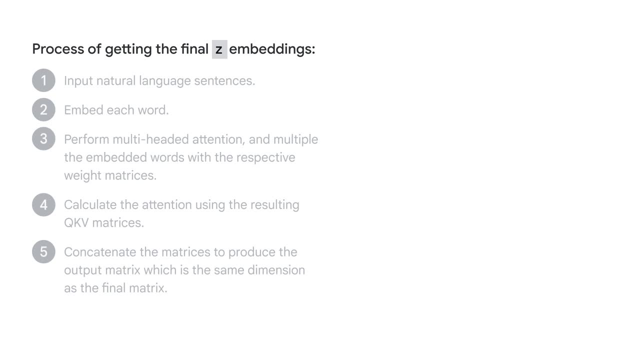 You can send along the resulting vector to the feedforward neural network. To sum up this process of getting the final embeddings, these are the steps that we take. We start with the natural language sentence, embed each word in the sentence. After that, we perform multi-headed attention eight times, in this case. 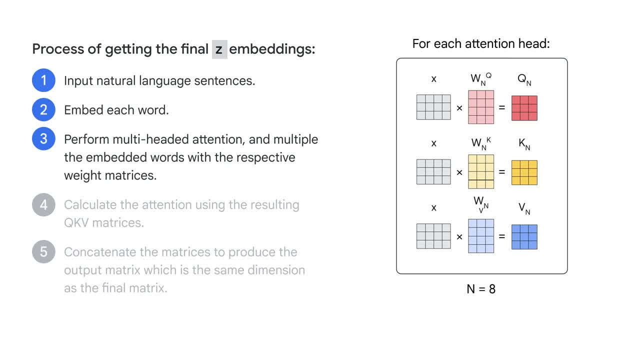 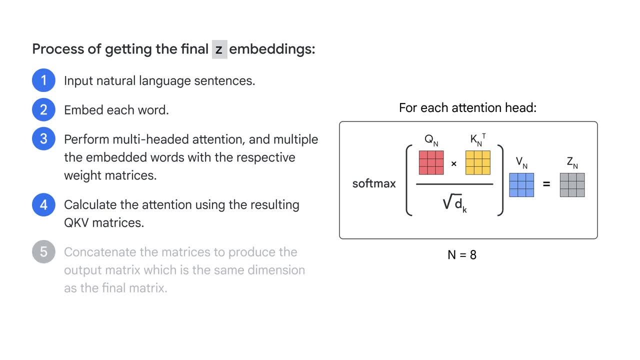 and multiply this embedded word with the respective weighted matrices. We then calculate the attention using the resulting Q matrices. Finally, we concatenate the matrices to produce the output of the self-attention layer. This is the output matrix, which is the same dimension as the final matrix that this layer initially got. 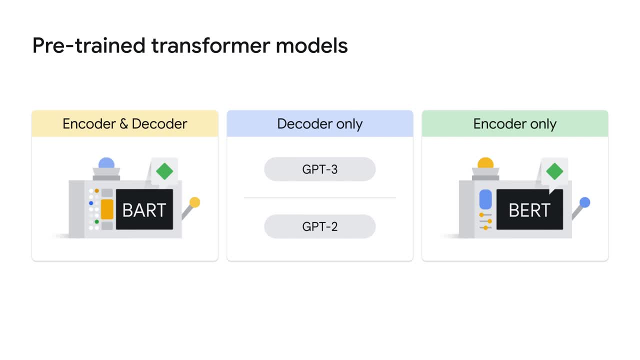 There's multiple variations of transformers out there now. Some use both the encoder and the decoder component from the original architecture. Some use only the encoder and some use only the decoder. A popular encoder-only architecture is BERT. BERT is one of the trained transformer models. 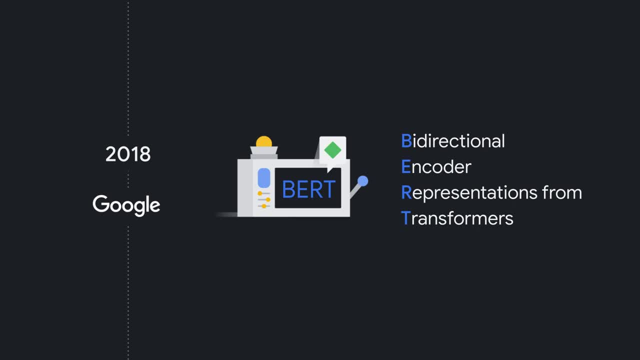 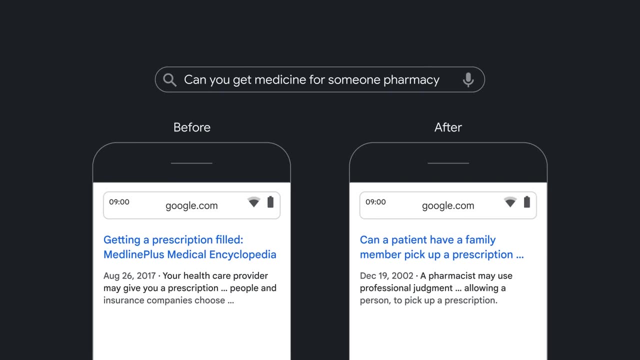 BERT stands for Bidirectional Encoder Representations from Transformers and was developed by Google in 2018.. Since then, multiple variations of BERT have been built. Today, BERT powers Google Search. You can see how different the results provided by BERT are for the same search query before and after. 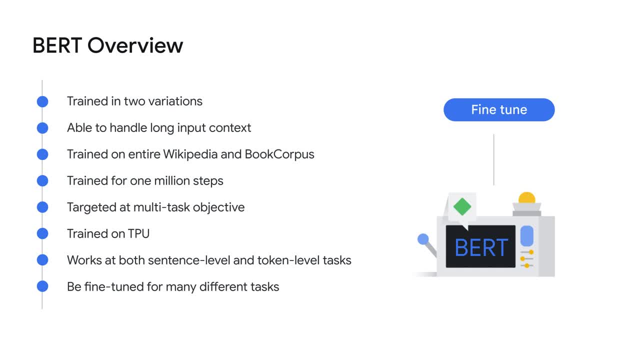 BERT was trained in two variations. One model contains BERT base, which had 12 stack of transformers with approximately 110 million parameters, and the other BERT large, with 24 layers of transformers with about 340 million parameters. The BERT model is powerful because it can handle long input context. 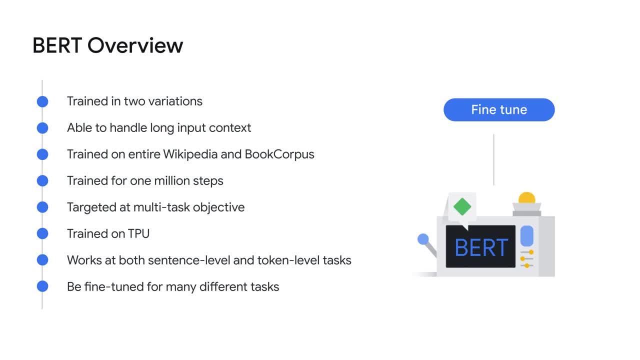 It was trained on the entire Wikipedia corpus and Books corpus. The BERT model was trained for 1 million steps. BERT is trained on different tasks, which means it has multi-task objective. This makes BERT very powerful Because of the kind of tasks it was trained on. it works at both a sentence level and at a token level. 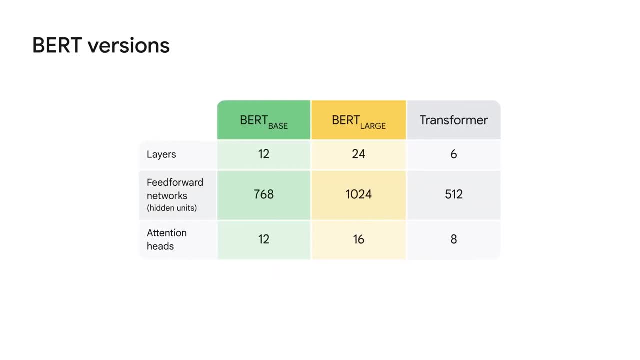 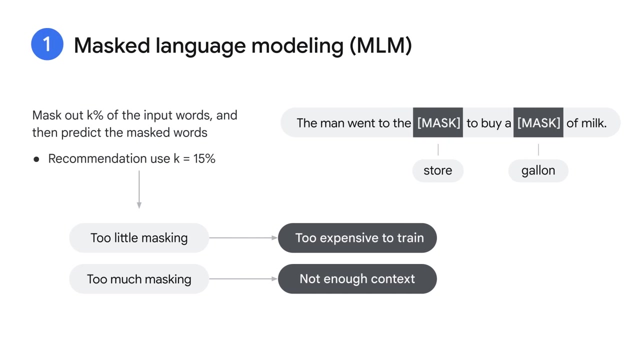 These are the two different versions of BERT that were originally released. One is BERT base, which had 12 layers, whereas BERT large had 24 layers, and compared to the original transformer, which had 6 layers. The way that BERT works is that it was trained on two different tasks. 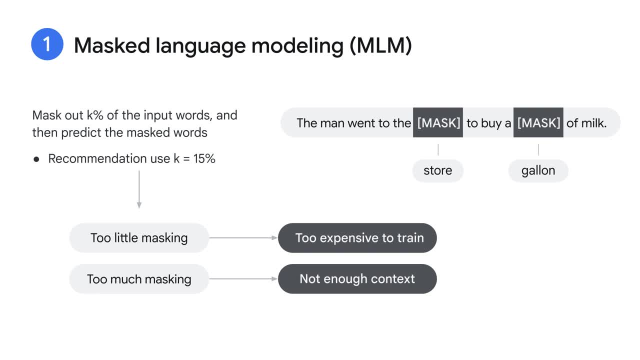 Task 1 is called a masked language model, where the sentences are masked and the model is trained to predict the masked words. If you were to train BERT from scratch, you would have to mask a certain percentage of the words in your corpus. 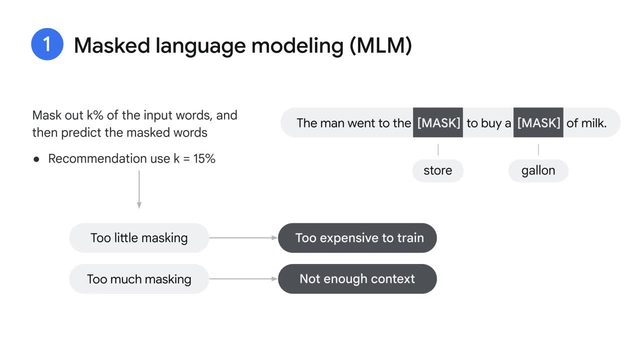 The recommended percentage for masking is 15%. The masking percentage achieves a balance between too little and too much masking. Too little masking makes the training process extremely expensive and too much masking removes the context that the model requires. The second task is to predict the next sentence. 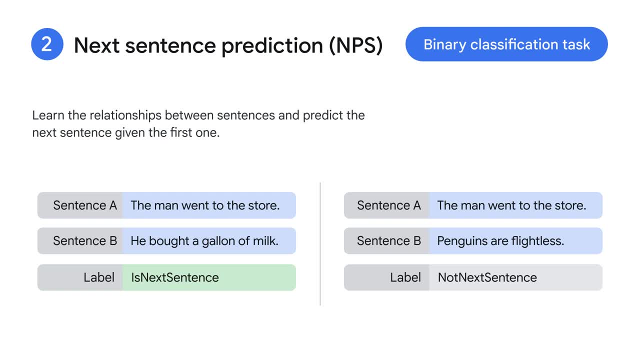 For example, the model is given two sets of sentences. BERT aims to learn the relationships between sentences and predict the next sentence given the first one. For example, sentence A could be A man went to the store And sentence B is. 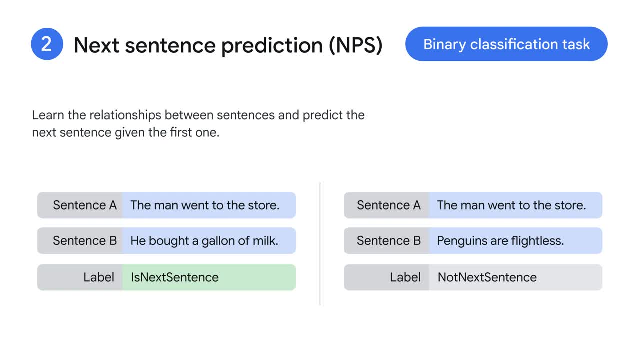 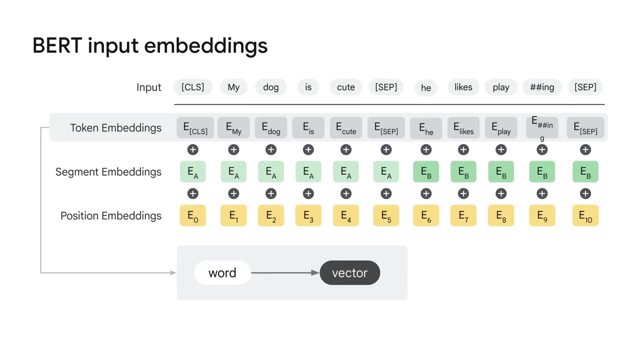 He bought a gallon of milk. BERT is responsible for classifying if sentence B is the next sentence after sentence A. This is a binary classification task. This helps BERT perform at a sentence level. In order to train BERT, you need to feed three different kinds of embeddings to the model. 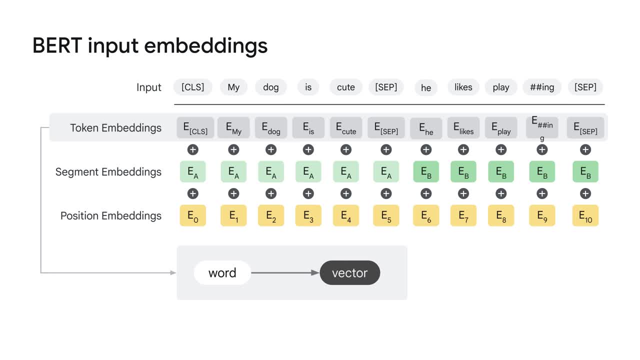 For the input sentence. you get three different embeddings: token, segment and position embeddings. The token embeddings is a representation of each token. as an embedding in the input sentence, The words are transformed into vector representations of certain dimensions. BERT can solve NLP tasks that involve text classification as well. 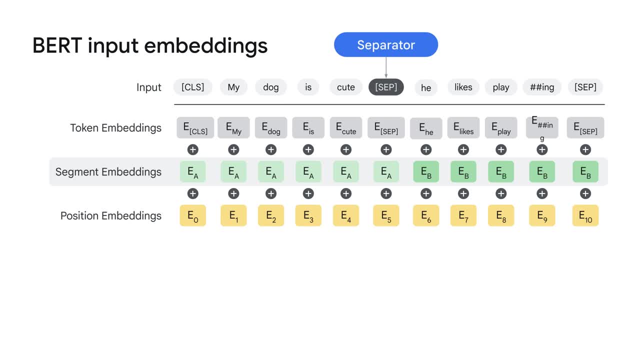 An example is to classify whether two sentences- say My dog is cute and he likes playing- are semantically similar. The pairs of input texts are simply concatenated and fed into the model. How does BERT distinguish the inputs in a given pair? The answer is to use segment embeddings. 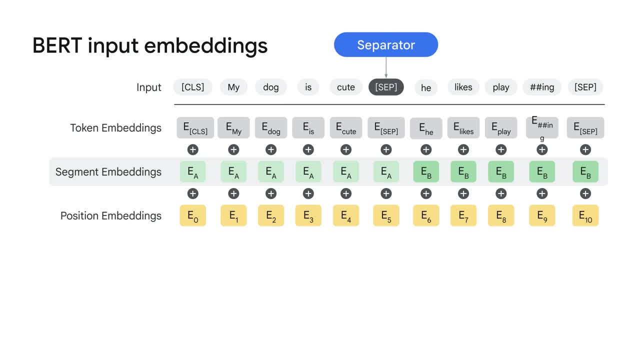 There is a special token represented by SEP, that separates the two different splits of the sentence. Another problem is to learn the order of the words in the sentence. As you know, BERT consists of a stack of transformers. BERT is designed to process input sequences up to a length of 512.